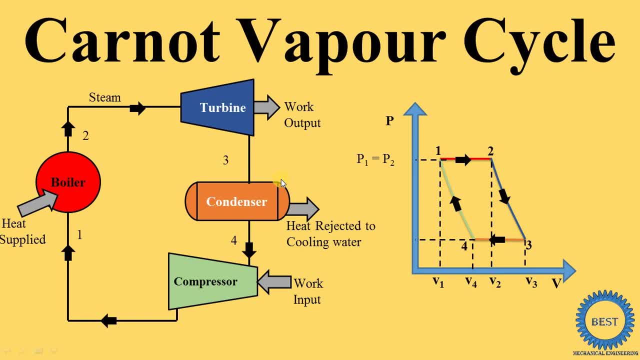 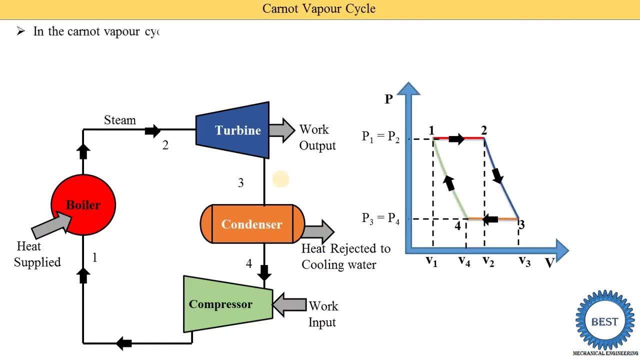 equations of the efficiency for Carnot vapor cycles And then, after I discuss the limitations of the Carnot vapor cycles. So in the Carnot vapor cycle steam or any other vapor is used as a working substance. in a place of perfect gas Means working substance in the Carnot vapor cycle is steam or any other vapor is used as a working substance. Component and arrangement of Carnot vapor cycles. 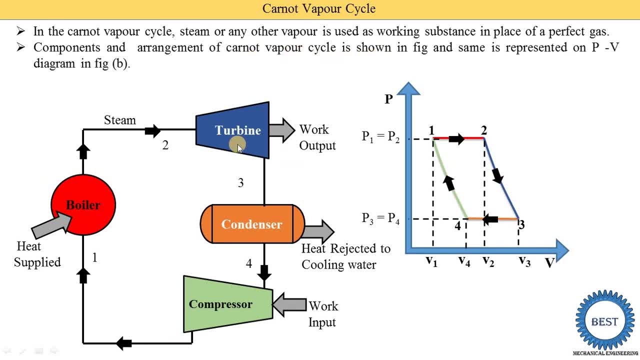 is shown in this figure. So in this figure you see these are the various components and arrangement of the Carnot vapor cycle. First component is boiler. Second is turbine, condensers and compressors. And same is represented on the PV diagram in this figure B. So this is the PV diagram and the various processes drawn here. So now we are understand the what is the functions of boiler, what happened in the boilers and how to draw the boiler process on the PV diagram. Then, after we understand about the turbine, 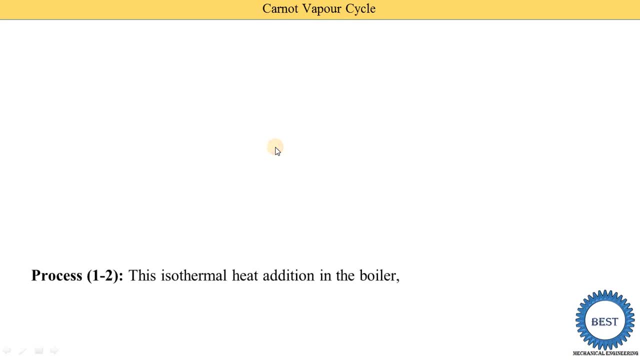 So you can understand the PV diagrams easily. So first process is the isothermal heat addition in the boiler. So this component is the boiler. Okay, So in a boiler we know the water is supplied and the water is converted into a steam. Okay, For converting the water into steam we require to supply some quantity of the heat. So we need to supply the heat energy to the boilers. and water is entered at the point one is converted into steam. 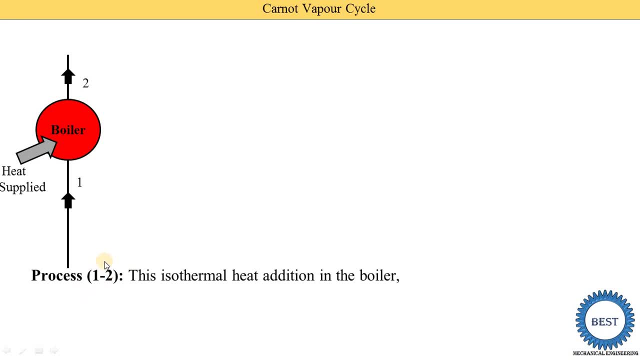 At the point two. So it is denoted as the process one to two, And here we mention isothermal heat addition. Isothermal heat addition means that temperature are not changed during this process. means the temperature at the one and two point are the same But only its phase are changed. means water is converted into the steam. So isothermal process having T1 and T2 is equal to constant. means temperatures before the boiler and temperature after the boilers are. 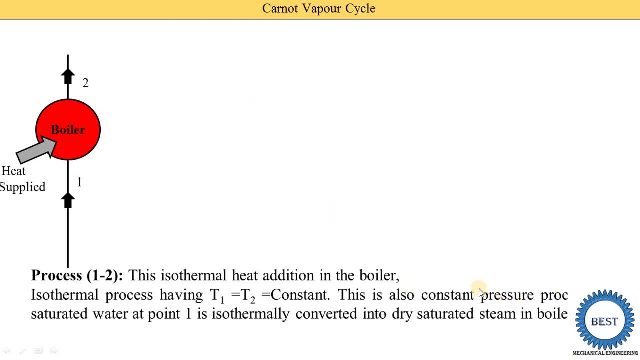 same. This is also constant pressure process. Saturated water at the point one is isothermally converted into dry and saturated steams in the boiler. means: at the point one the saturated water is there and it is converted into dry and saturated steam in the boilers. Now we draw this one to two process on the PV diagram. So on the y axis, pressure is there. on the x axis, volume is there. So at this point, the value of the 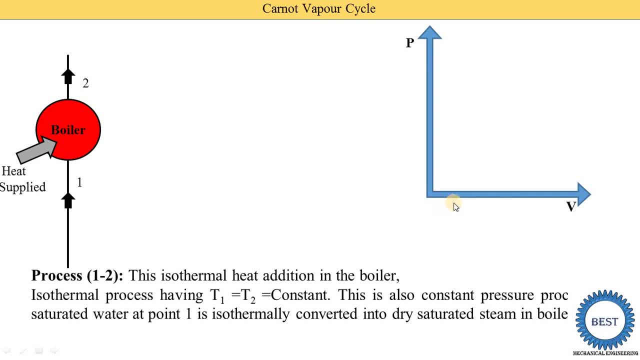 pressures and volumes are zero. okay. so when we moving right side on the x-axis, the value of the volume is increased. okay. when we moving on the upper direction on the y-axis, value of the pressure is increased. okay. so in the boiler, what happened? that is, a isothermal heat additions with the. 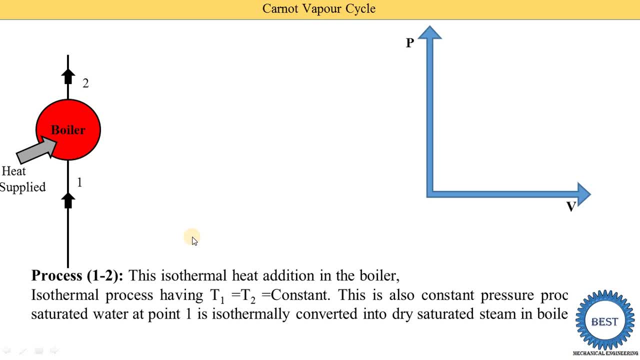 isothermal heat additions, the pressure of the water is also remains constant, okay, and when water is converted into the steam, its volume is increased, okay. so suppose this is the point number one, because in a boiler highest pressure is there, okay, so we need to draw this one point. 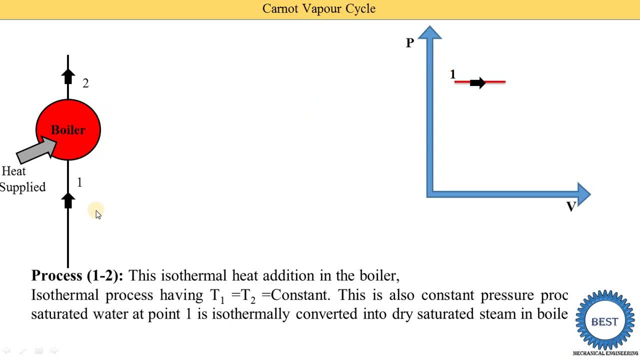 on the upper side and the volume is increased during conversions of water into steam means v1 is greater than the v2s. that's why we need to move towards the right sides. okay, so here you see it is. the p1 and p2 are same means. in a boiler pressure is remains constant. here the v1 volume. 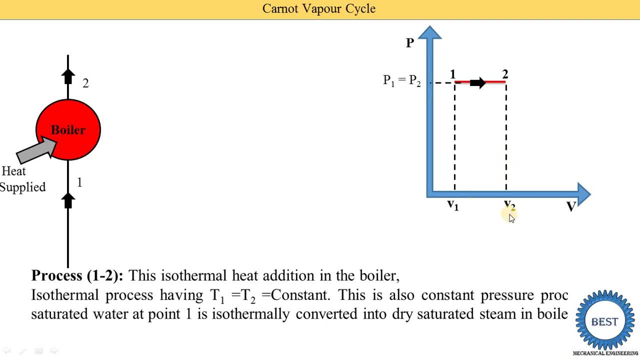 here the volume, v2. volume means this v2 is higher than the v1. second process is the process two to three. this is the reversible adiabatic expansion of the steam in a turbine means next component is the turbine. so here you see, this is the turbine. okay, in the turbine we supply these teams and the steam. 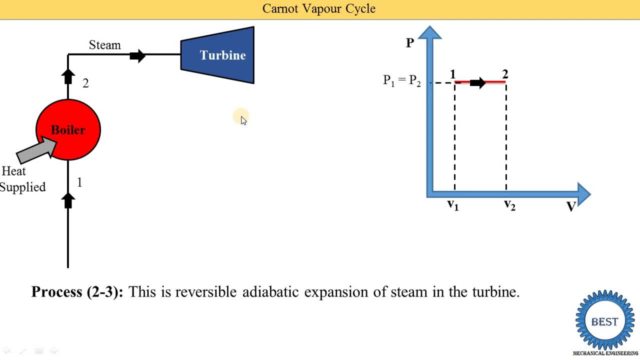 is produced. some mechanical work means this steam is supplied on the blade of the turbine. the turbine will start to rotate. okay, so this heat energy is converted into the mechanical energy in the turbine. means turbine is give some work, output. okay. so in a boiler we supply some quantity of heat, in a turbine we get some amount of the work done and it is the. 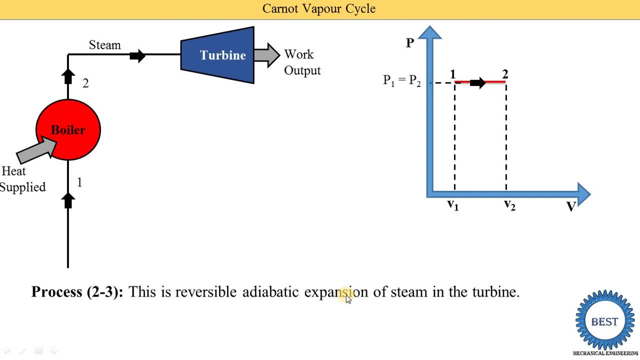 reversible adiabatic expansion. expansion means the pressure is reduced and volume is increased. sorry, pressure is reduced and volume is increased. it is called as the expansion process. okay, the dry steam at the point 2 is expand adiabatically in a steam turbines and develop the work and this work. 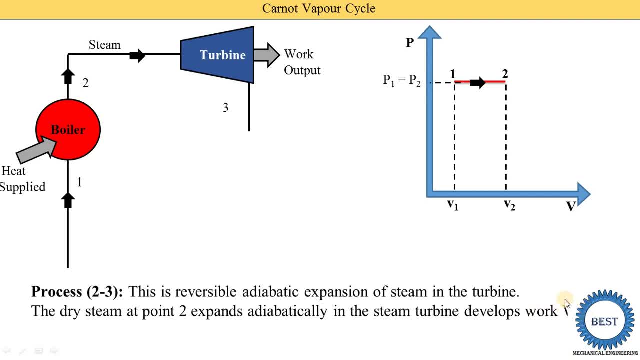 is denoted as the wt. okay, w means work and t means turbine. okay, so how we draw these two to three lines so we know that the pressure is reduced in the turbine, okay, so this point number three is moving in the downward side. but point number three is coming either on the left side or a right side. 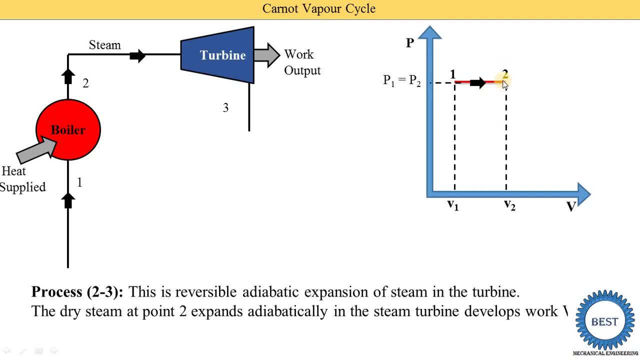 compared to the point two. so we know that during the expansion volume is increased. okay means v3 is higher than the v2. then we need to move towards the right sides and the pressure is reduced means we need to move towards the downside compared to the p2 means we are getting the three points. 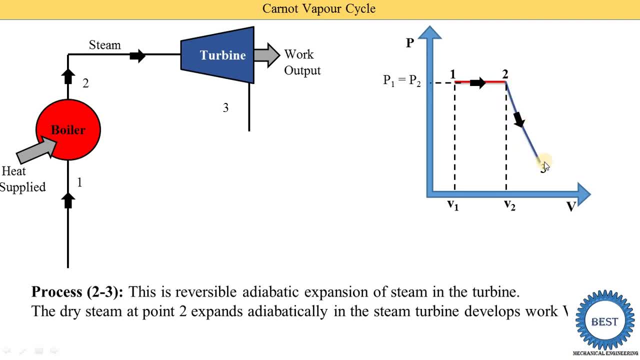 somewhere here. okay, and we need to draw this type of the cow line. so here you see, there is a p3, pressure is there. so p3 is lower than the p2 and this v3 are higher than the v2. now the next process is the process three to four. it is the isothermal heat rejections in the 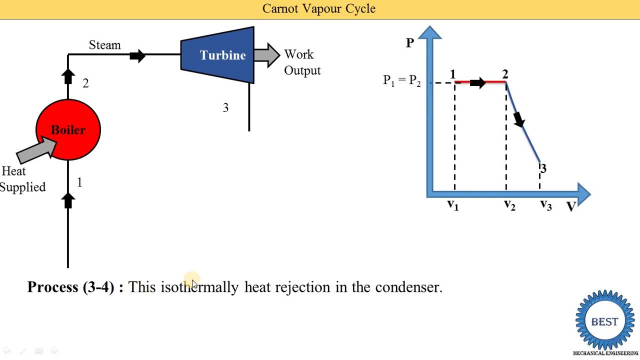 condenser. so three to four process is the heat rejection process, okay, and this heat rejection is done in the condenser. okay. so in a first component- boiler, you see, that is- the heat is supplied. okay, now this heat is rejected in the condenser. so here we draw the condensers. okay, and 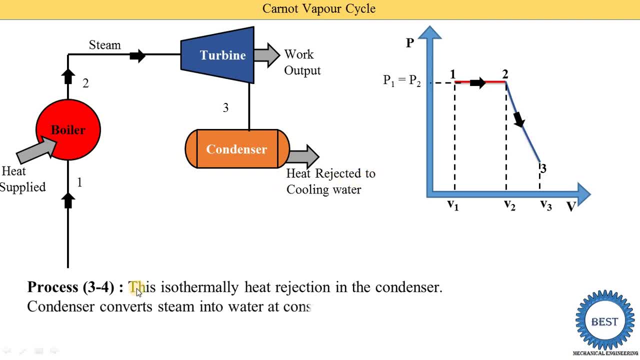 in the condenser, heat is rejected to the cooling waters. so condenser is convert steam into water at the constant pressure and the temperature as shown in the diagrams. okay, so functions of the condenser is that we reject the heat and when we reject the heat, the steam is converted into the. 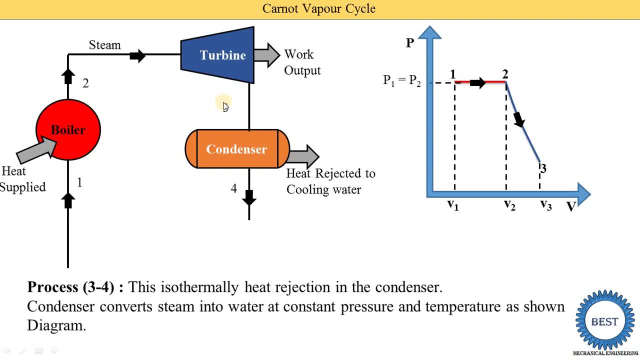 water. so this process is three to four. at the point number three, that is a steam, and at the point number four, water is there, okay. and during that process the pressure is remains constant. so when the pressure is remains constant we need to draw the horizontal line, means p3 and p4 are 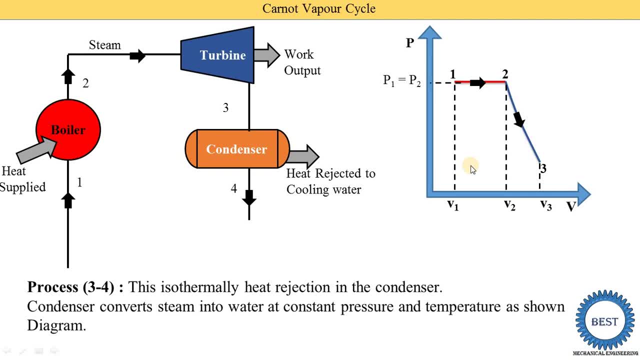 same. so when the heat is reject, so steam is converted into water, means gas is converted into the liquid. that means the volume is reduced. okay, the volume is reduced means at the point three, we have the two option: either we move towards this side- means right side- or either we move towards the left side- okay, but we know that the volume 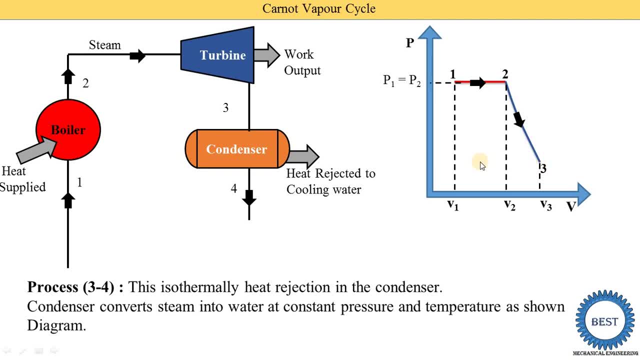 is reduced. so when the volume is reduced we need to move towards the left side, means the point number four is coming left side compared to the point number three. so this type of the line we draw horizontals and here the point number four. so here we indicate that it is the v4. 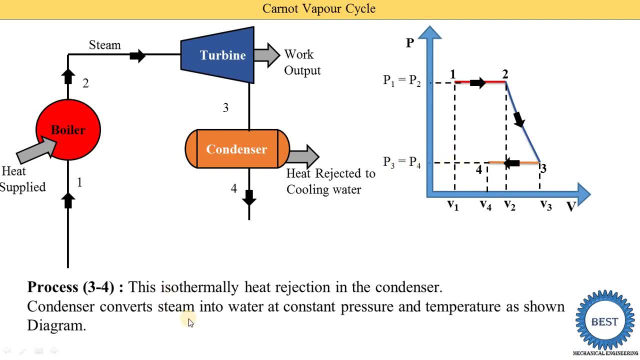 and here we indicate the p3 is equal to p4, because we have written that the constant pressure process and the temperature is also constant. okay, that is isothermal heat rejection. isothermal heat rejection means when we draw the ts diagram: okay, so three to four process are drawn the horizontals. so at the completing the four, 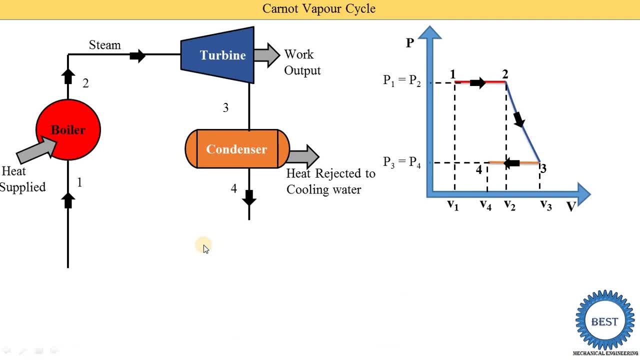 process. i also show you the ts diagram. at that time you can clear your concept. now, process four to one. this is the reversible adiabatic compression process- means we need to do compression process and for do the compressions we require the compressor. so here component four. 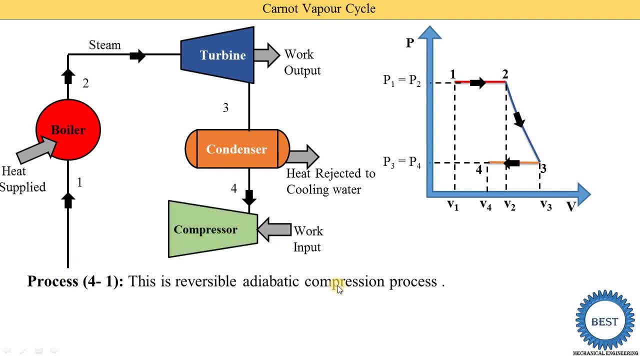 is the compressor, and in the compressor we need to supply some work input. okay, so here you see, in the second component means turbine. turbine is produced, some work done, and the compressor is consumed, some work input. so it is the process four to one, so steam and water enters into the 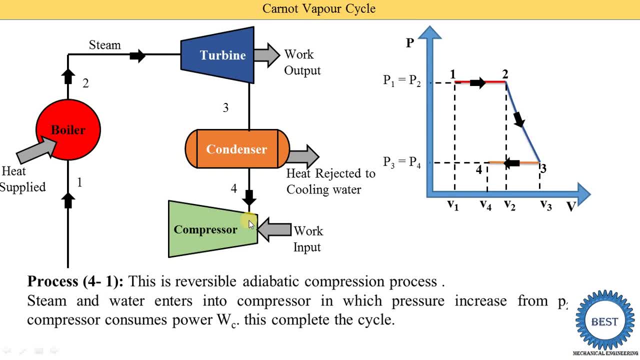 compressor means at the point number four. it is not necessary. at the point number four it is a completely water state. is that some particles of the steam is also there? okay, so steam and water enters into the compressor, in which pressure is increased from p4 to p1 and the 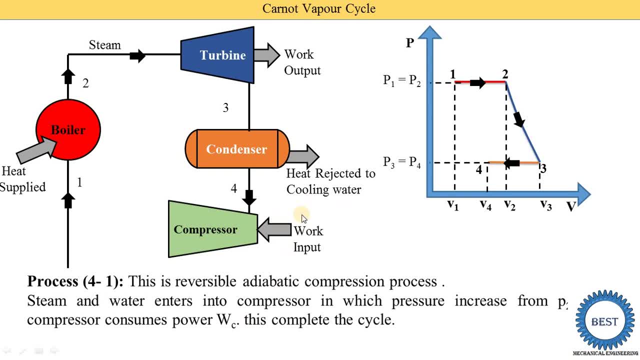 compressor is consumed. some power means say they consume some work, so it is denoted as the wc and this complete the cycles. okay, so here we close it to the point number one and outlet of the compressor. so cycle is completed. now how to draw this line on the pv diagram? so just we need to. 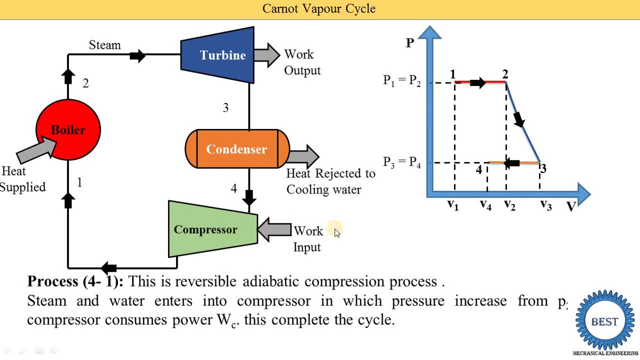 connect this four to one line. okay, so in a compressor we know that the pressure is increased and the volume is reduced during the compressions. so when the pressure is increased the point number one is moving in upper direction compared to the point number four, and on the x axis they are moving on the left side because the volume is reduced. so we draw this type. 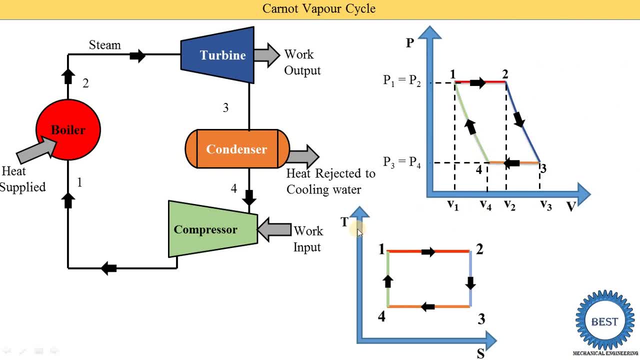 of the lines. okay, now, here you see, this is the ts diagrams. okay, so what? we study the heat supplied and the heat rejections are carried out at the constant temperature. so here you see, we draw the description of the temperature corresponding to the temperature. so we take this asussian heat. 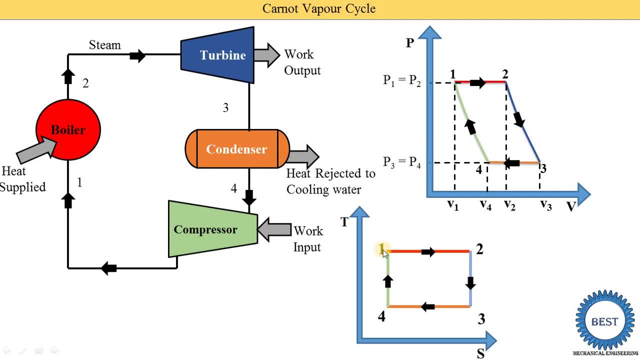 addition, and we draw, the temperature is constant. so when we take the projections of this point one and point two on the y-axis, we get the same point, which is: t1 is equal to t2. inter turbine temperature is reduced at the constant entropy. so we draw this type of the downward line because 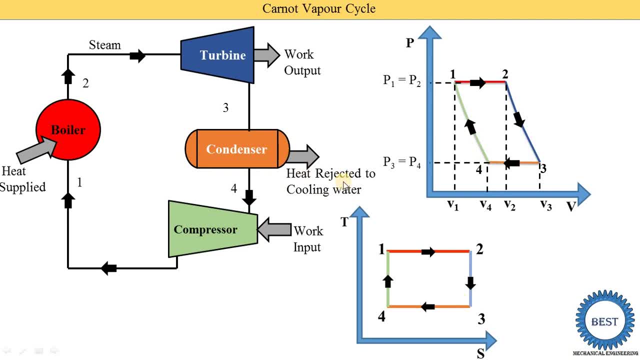 temperature is reduced and entropy is remains constant. in a condenser, heat is rejected means heat is rejected at the constant temperature. means t3 and t4 are same. okay, just team is converted into water, but its temperature are same. that means we draw the horizontal line, so we take 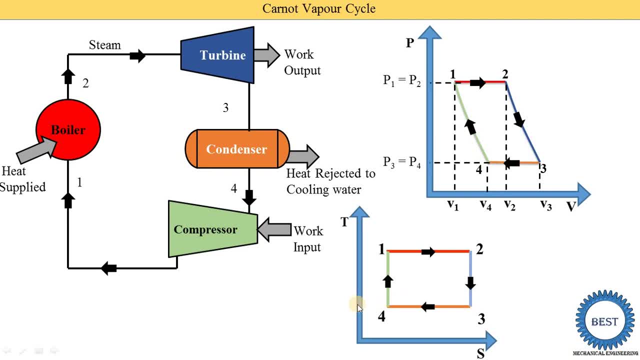 the projections of the 0.3 and 0.4 and the y-axis, we get only one point: means t3 is equal to t4 and in the point in a compressors we supplied some work, input means this work is converted into the heat, means its temperature is increased and the entropy is remains constant. now next, we 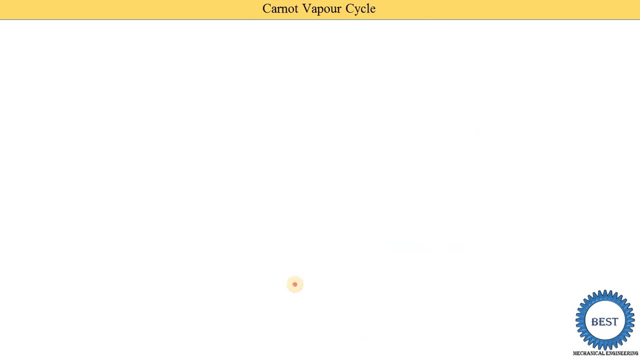 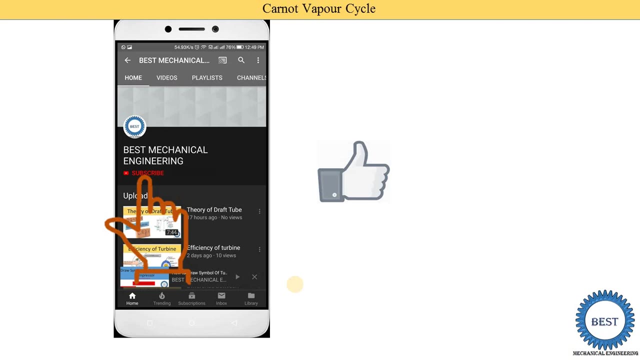 derive the equations of the Carnot vapor cycles. okay, now, before moving it, I request to like the video and subscribe my channel for watching the more video related to the BME and other subject of the mechanical engineering. for the BME or EME subject. various link is provided in descriptions. 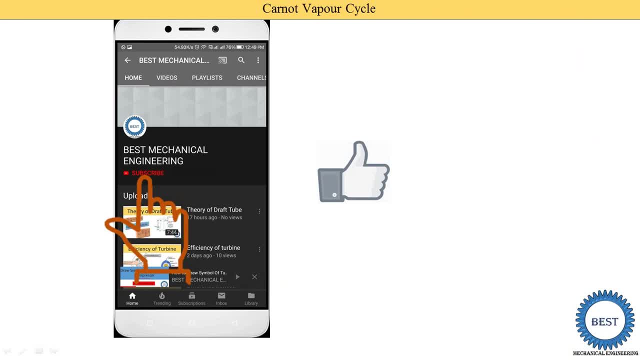 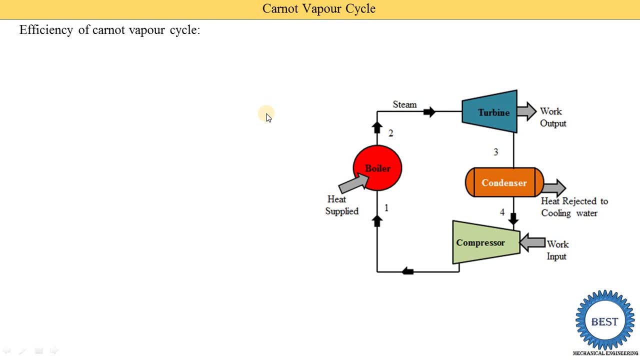 as well as in a card card, mean on a top right screen of your mobile or laptop. you see the i symbols. now, here we derive the equations of the efficiency then, after we study the limitations. so what is the equation of efficiency of Carnot vapor cycle that we derives? okay, 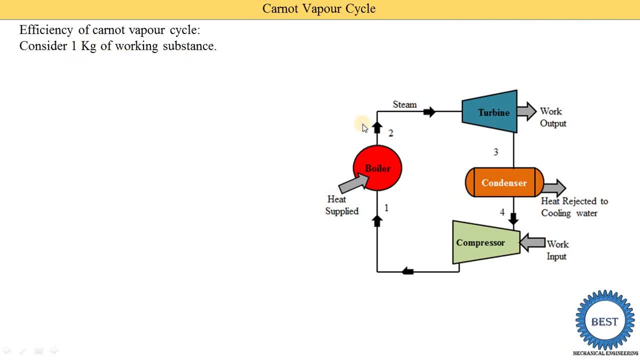 for that we consider the 1 kg of working substance is there. you can see that we have 1 kg of working substance is there, so we can derive the efficiency of Carnot vapor cycle. that means we are considering that the steam is produced 1 kg and according to the 1 kg of. 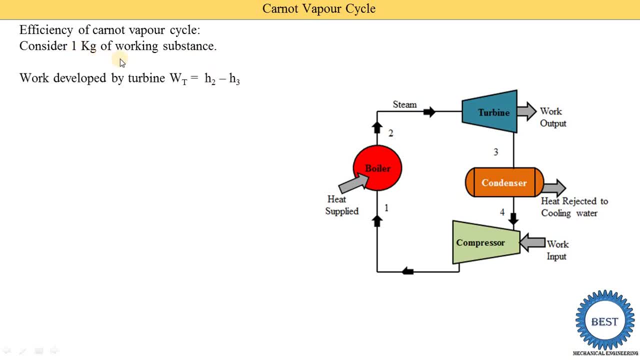 the mass of water for a mass of streams. we find out the equations of efficiency. so we know that this turbine is produced. some work done, okay. so how amount of the work done is produced by the turbine? there is a word developed by the turbine. it's denoted as the w? t. okay, so here. 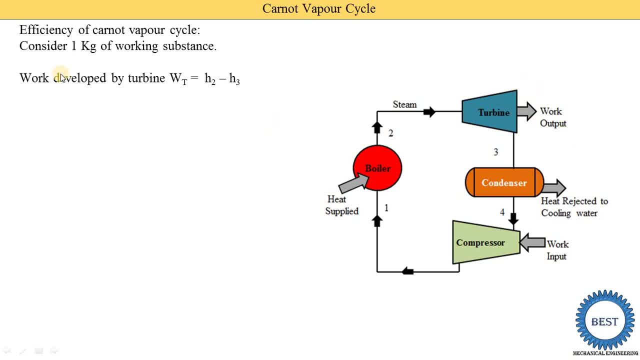 you see, we indicate work output. so this work output is called as the work developed by the turbine and it is denoted as the w, t, w means work and t means thermal work. so here you can see the turbine and in the turbine process is two and three. okay, so we return enthalpy, h2 minus enthalpy. 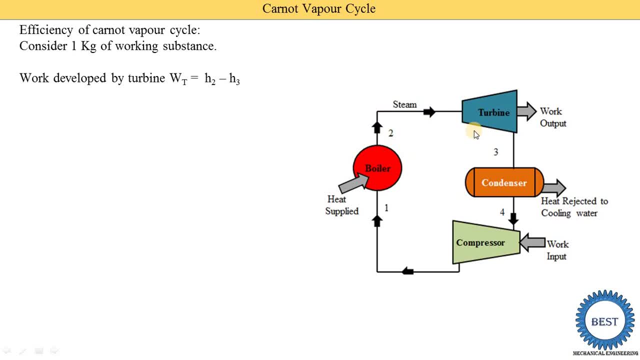 at three because the steam have the higher enthalpy. at the point two then the enthalpy is reduced. why this reduce? because the energy in the steam is used to produce some work done. okay, that's why its energy is reduced. so at three is lower than the h2. that's why we return h2 minus at three. 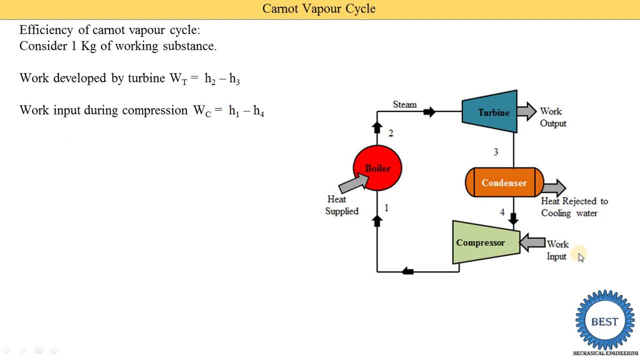 second, work input during the compression. so here in this compressor you see we need to supply some work done. so how amount of the work done we supplied, that is find out by using these equations. okay, so this work input during the compression is denoted as the wc. w means work. 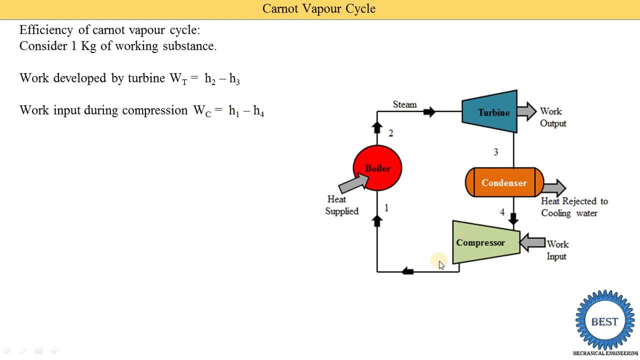 c means compression. it is denoted as the h1 minus h4. so here h1 is higher because the water coming at the four point. so in this water we supply some work. so this work is added means h1 is higher compared to the h4, so it is written h1 minus h4. so net work developed means in one component we 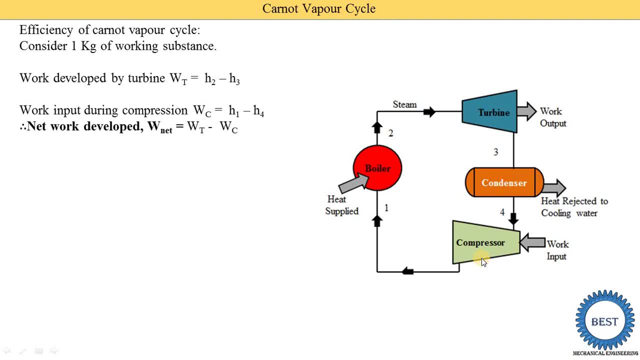 produce some work done. so in this water we supply some work. so this work is added means h1 is higher, is work done, and in a compressor we supply somewhat. that means work. output from the component is positive, work input to the component is negative. that we already study in a chapter. 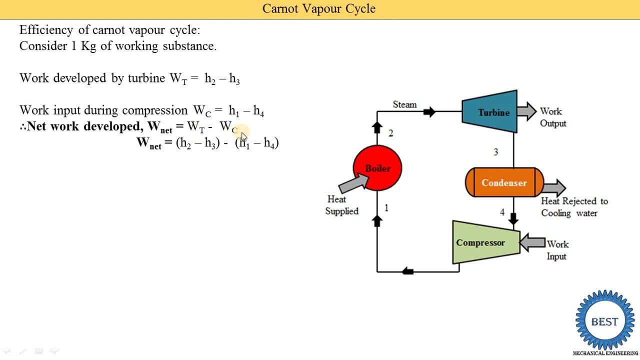 number one. okay, so net work is the wt minus wc. means turbine is produced work. it is considered as the positive. in a compressor we supply work done, then it is considered as the negative. okay, we have the equation of wt and wc. so it is written: h2 minus f3, bracket over 100 bracket. h1 minus h4. 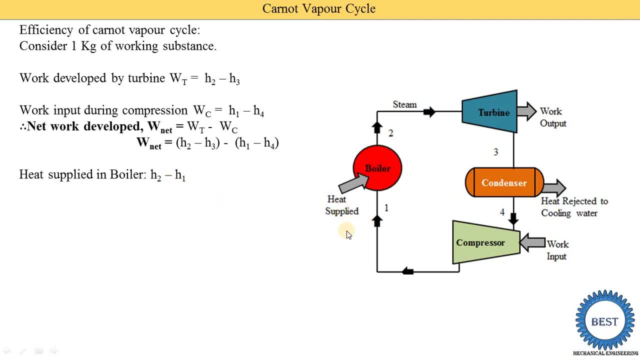 now next, heat supplied in the boiler. so in a boiler, how amount of the heat is supplied? so in a boiler we supplied the h2 minus h1 quantity of the heat. so at the point one water is coming in a water, we heat, we supply the heat. energy means h2 is higher compared to the h1. so 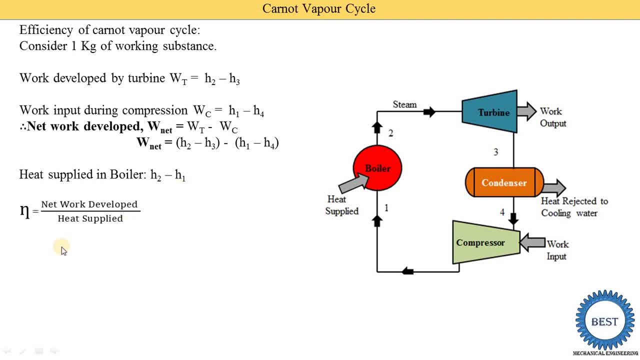 it is written h2 minus h1. now what is the equations of efficiency? so efficiency is equal to network developed divided by heat supply. so equation of the efficiency for the any system is output upon input. what is the output? output is in the form of the work, because the carnot vapor 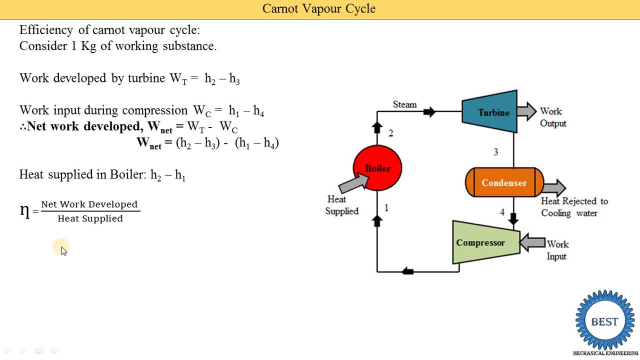 cycle is one type of heat engine. so in a heat engine, work is output, heat is supplied. so what is the output? work? it is the w net, okay, and this is the equation. and what is the energy? what is the input? input is the heat supply to the boiler, okay, so we putting this value. network developed is h2. 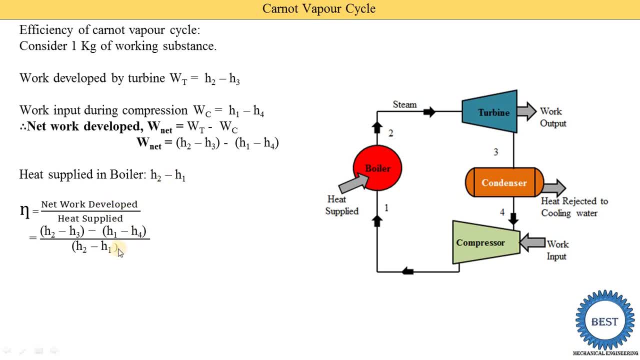 minus f3. another bracket, h1 minus h4- heat supply- is h2 minus h1. now in this equation we do the same, okay, what we do. this h3 is going this bracket and h1 is coming in this bracket. okay, so here we return: h2 minus h1. this h3 is going on this side, so it is h3 minus h4. okay, now, then after. 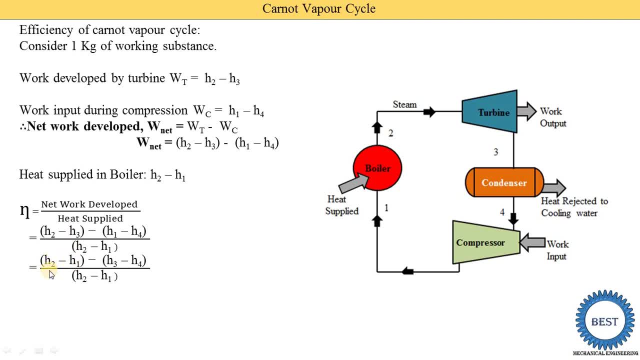 we divide this equation in a two parts, that is h2 minus h1, divided by f2 minus h1 minus second side, that is at 3 minus h4 upon h2 minus h1. so we get this type of the equation because this part is cancelled, that is h2. 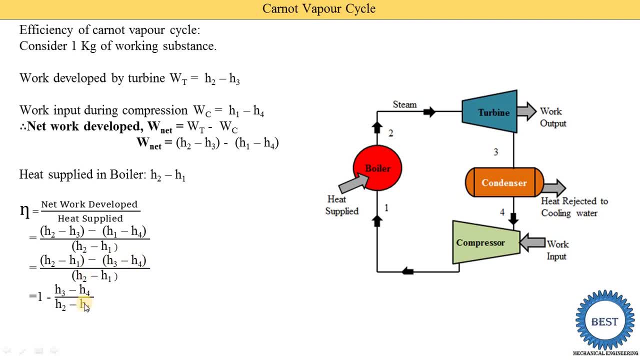 h1 is 1. second part is h3 minus h4 divided by h2 minus h1. so this is the equations for the efficiency of the Carnot vapor cycles. now we know that the h3 minus h4 is denoted as the heat rejected by the condenser. okay, what is suppose we consider here? three point, and this is four point. 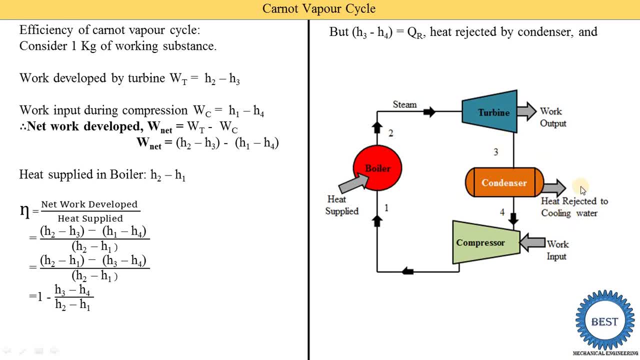 so what this h3 minus h4 is given, that is, the heat rejected by the cooling water, means instance of this h3 minus h4. we are able to return the qr, that is, the heat rejections, and instance of this h2 minus h1. we know that this is the heat supplied to the boiler. 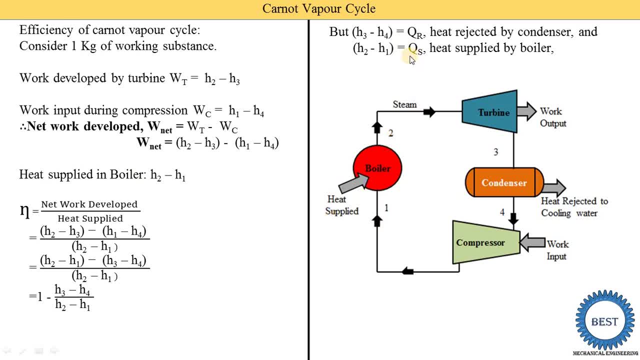 see this: h2 minus h1 is equal to the heat supplied to the boiler. that is denoted as the qs. so q is indicate for the heat, r is indicate rejections and s is indicate the supply. so we modify these equations. efficiency of Carnot: vapor cycle: that is the 1 minus heat rejection divided. 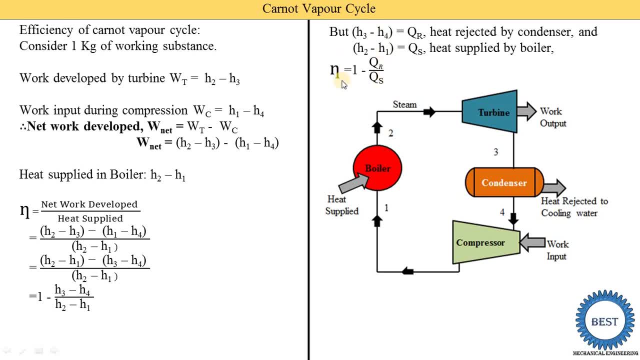 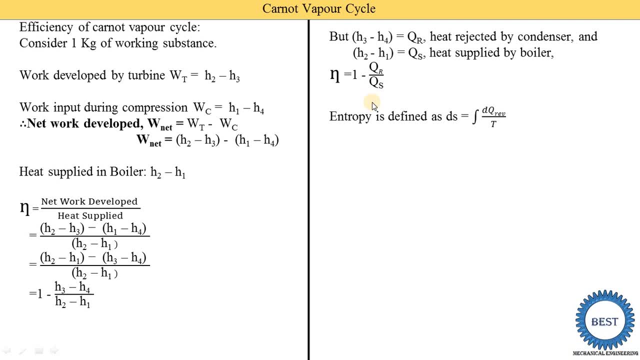 by heat supply. okay, so this is the another equations of the Carnot vapor cycles. now we further solve this you equations by using this ts diagrams. okay, so we know that entropy is defined as ds integrations: change in the heat energy reversible divided by temperature. so we can write: 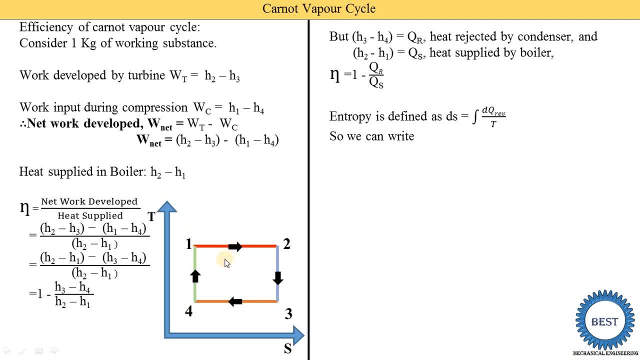 means from the ts diagram what we write: okay. so in a one to two process- this we know, that is, we are supplying some quantity of the heat energy, okay. and during three to four process we are rejecting some heat energy, okay. so first we make the equations of the qr from this ts. 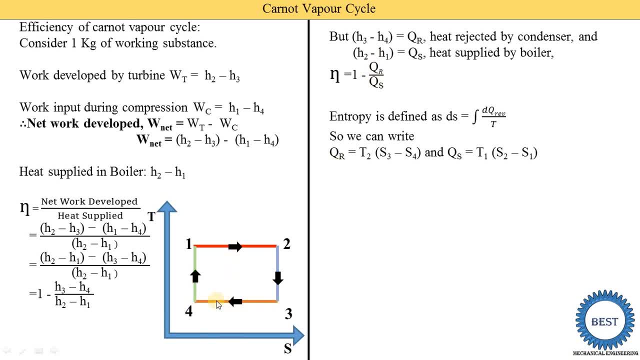 diagram. okay, so this area below this three to four line is indicate the heat rejection. okay, so we are getting one rectangle. okay, so in a rectangle, what is this height? so this height is the t3. okay, but we are considered only two temperature: this is the t1 temperature and this is the t2 temperature. 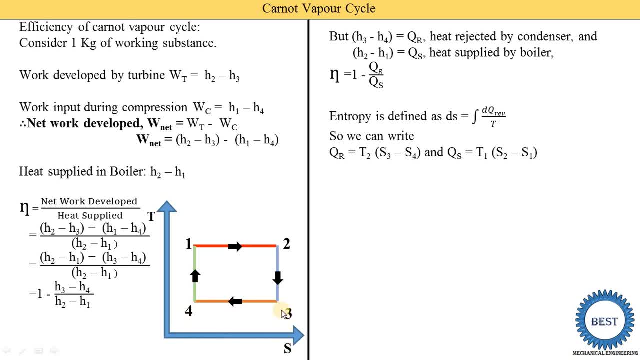 so we draw one rectangle here. then we get the height of the rectangle is t2- okay. instance of this trait: we consider it is the t2- okay. so in a rectangle we get height is htn- okay. so we are drawing a rectangle here, okay, and there is one height inside. so we draw here, we use 3t and we 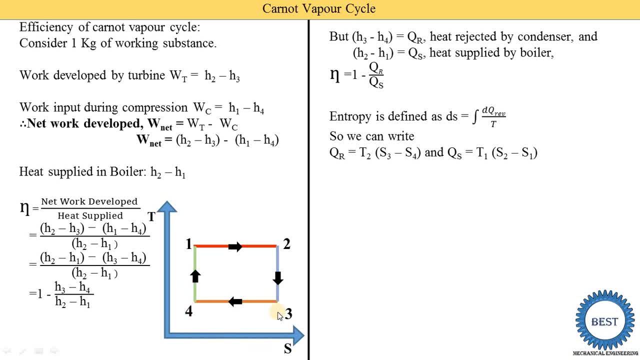 okay, and what is the width of this rectangle? it is the s3 minus s4, means thus we need to return this area of the rectangle, okay. what is the heat supply? heat supply is in the 1 to 2 process, means area below this 1 to 2 line is considered as the heat supply. okay, so what is this height? 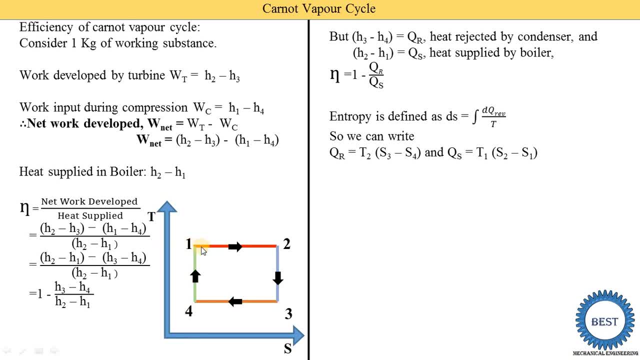 of this rectangle? it is the t1. okay, what is the width of the rectangle? it is the s2 minus s1. okay, so we can return this equation like this way. that is how we putting this value of qr from the ts diagram, it is t2. in bracket, s3 minus s4. we putting the value of qs, that is a t1. 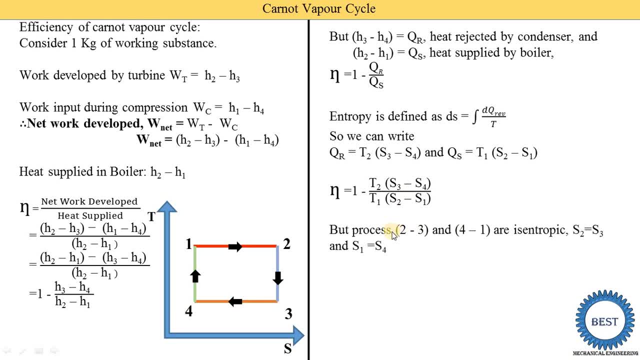 s2 minus s1, okay, but the process 2 to 3 and the process 4 to 1 are the isentropic. okay. so here you see. then we take this projection of the point 2 and 3 on the x-axis, we get that s2. 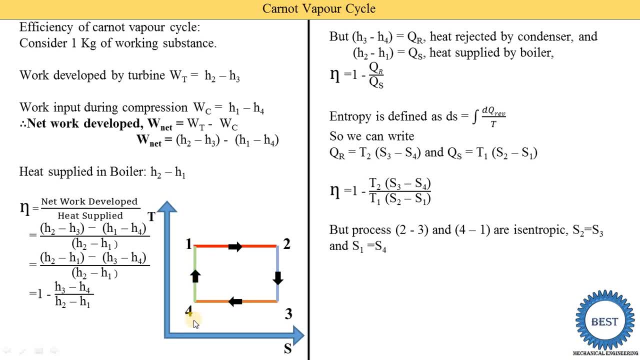 is equal to s3. we take the projection of 1 to 4 on the x-axis, we get the s1 is equal to s4. okay, means s2 is equal to s3. s1 is equal to s4. then suppose we putting this, s3 is replaced by s2. 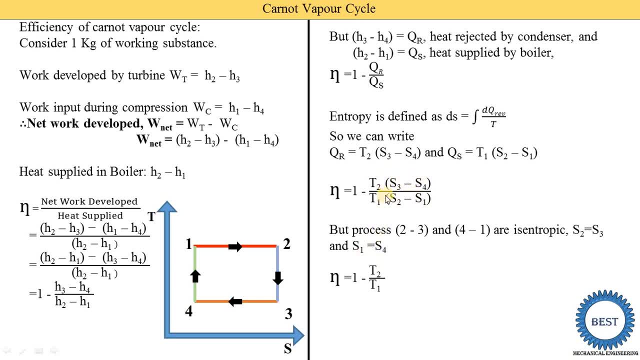 and this s4 is replaced by the s1, so we get the s2 minus s1 in a below part also s2 minus s1, though they are cancelled. so we get these simple equations for the Carnot vapor cycle. the efficiency is equal to 1 minus t2 upon t1. okay, so this is the final equations for the efficiency of Carnot vapor cycle. 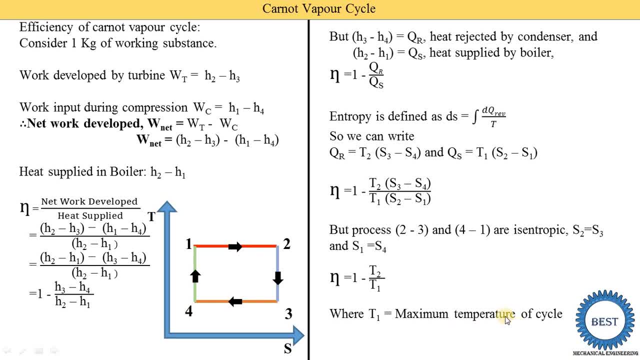 now what this t1 is indicate. t1 is indicate the maximum temperatures of the cycle and t2 is indicate the minimum temperature of the cycle. so here we only two temperature. this is the t1, and here t3, t4. so this is considered higher temperature and this is considered the. 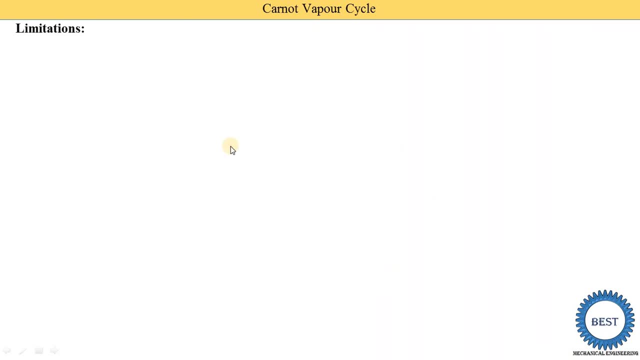 lower temperatures now. next, we understand the limitations of the Carnot vapor cycle. so in a Carnot vapor cycle we study the different four process. okay, so in a process four to one. what we study, so process four to one, it is in the compressors. okay, that is a adiabatic or isentropic compressions of the wet vapor. 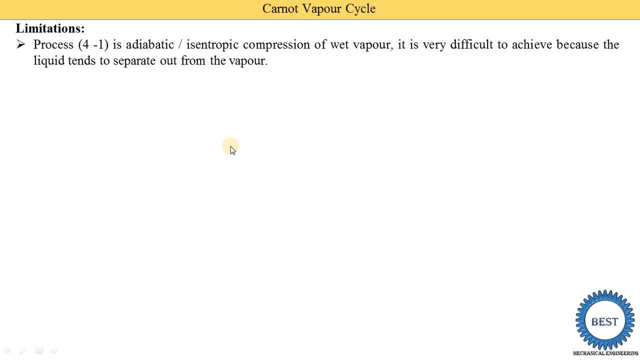 wet vapor means that is a water particle is there in the vapor, so it is very difficult to achieve because the liquid tends to separate out from vapors. means we know that we are not able to increase the pressure of the liquid particles into the compressors, so practically. 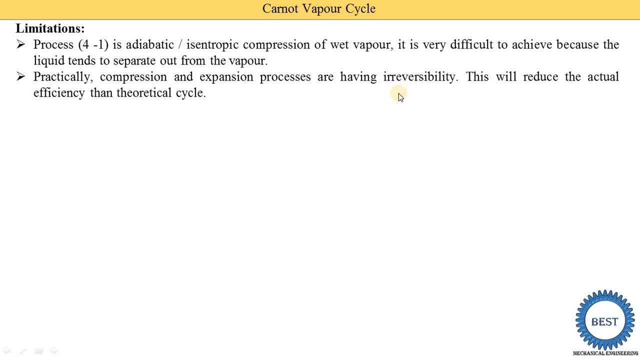 that's our process, that we know that the liquid particles like to blow onto it, so that's what we call average temperature. anything you have a heat transfer to aß through, it is a hot chamber and outside temperature, as you can see here, we have got an expansion followed by an increase. the thermal efficiency and acceleration process are having irreversibility, so these will reduce the actual efficiency than the theoretical cycles to achieve super heating of steam at the constant temperatures and the pressure has 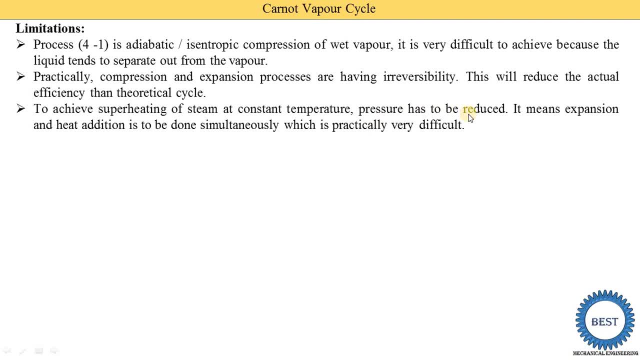 we do the superheating okay. so at the constant temperature pressure has to be reduced. it means expansion, and the heat addition is to be done simultaneously, which is practically very difficult. so these are the various limitations of the carnot vapor cycle. so this carnot vapor cycle is actually not possible and in this real life none of the any cycle.